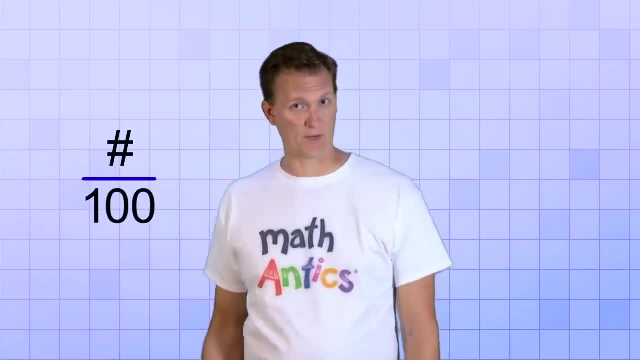 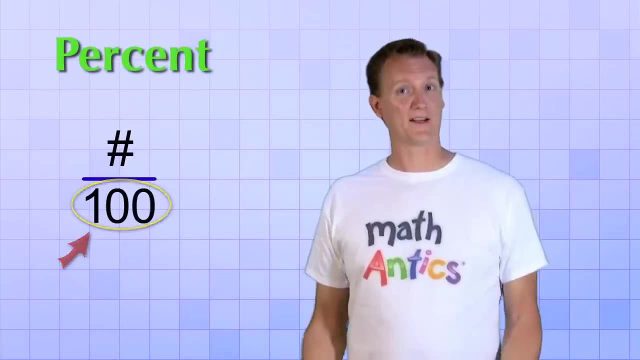 A percent is a special fraction that always has 100 as the bottom number. If it's a percent, then no matter what the top number is, the bottom number will be 100.. In fact, because the bottom number of a percent is always 100, we don't even write it. 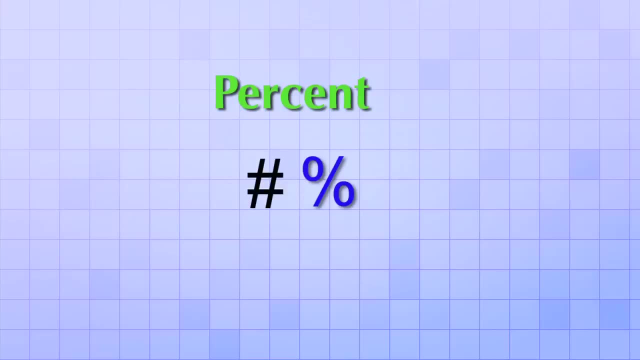 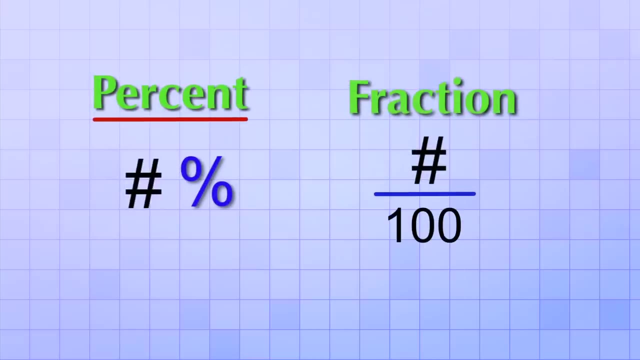 Instead, we use this handy little symbol called a percent sign. Whenever you see this symbol after a number, it means the number is a percent. It's really a fraction with 100 on the bottom, but it's just being written in this more compact form. 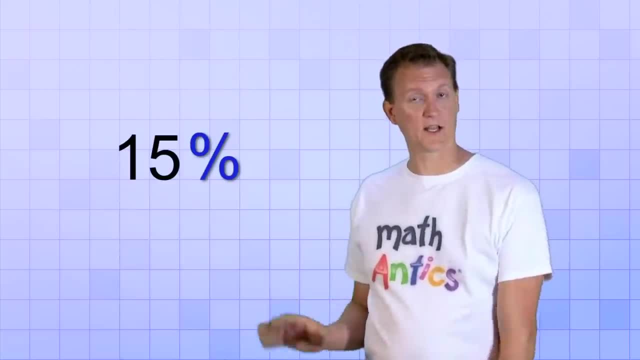 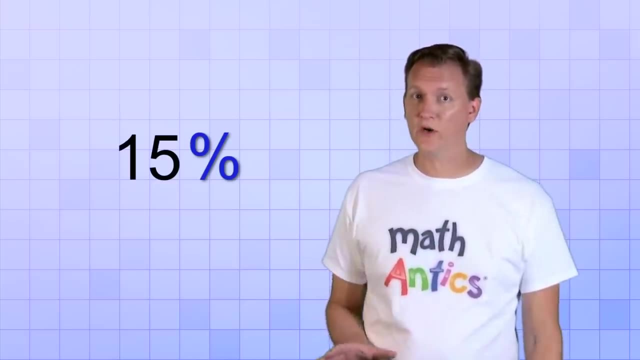 Like this number 15. here It's got the percent sign after it, so we read it as 15%, And because a percent is really a fraction that always has 100 as the bottom number, we know that it means the same thing as 15 over 100.. 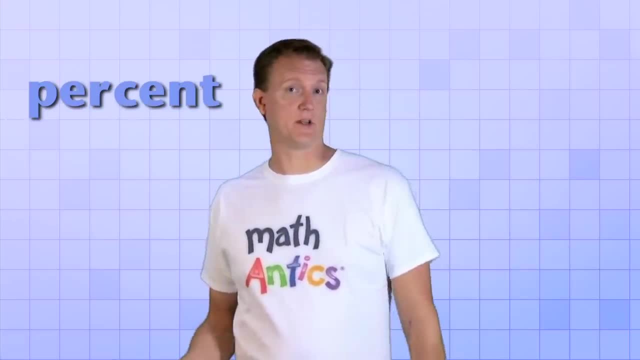 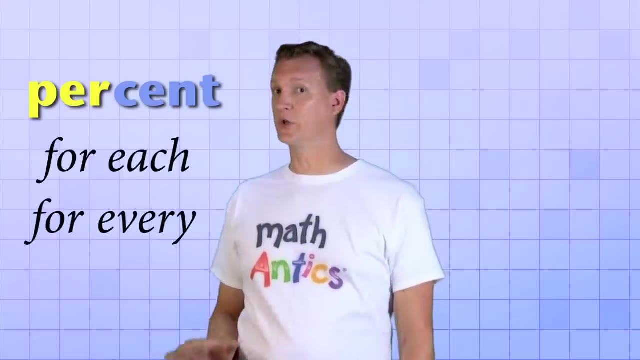 Percents make even more sense if you know what the word percent means. The prefix of the word per means for each or for every. You know like if someone said only one cookie per person And the root word cent is Latin for per. 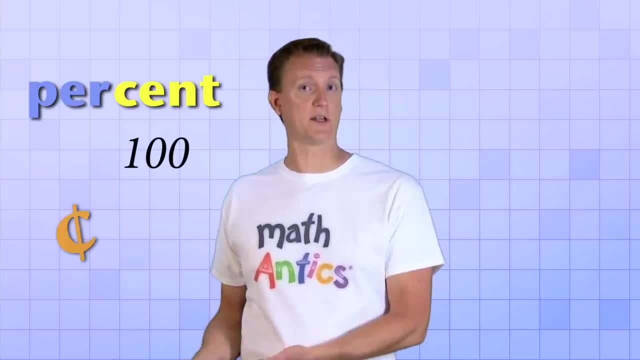 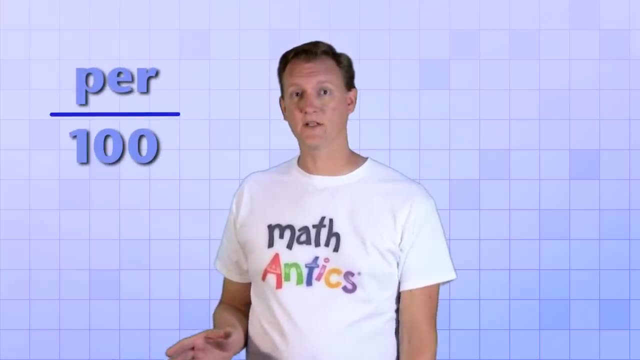 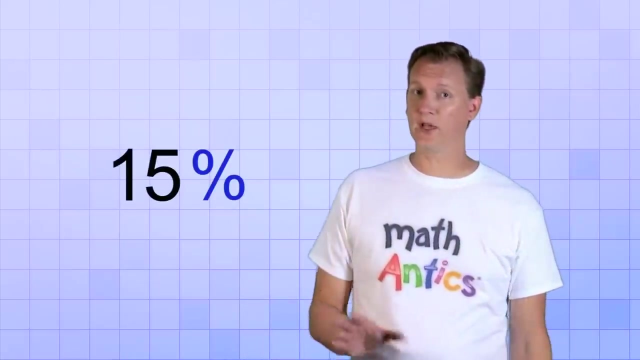 Cent is Latin for 100. That's why there's 100 cents in a dollar. So percent literally means per 100. And that's why there's shortcuts for writing fractions that have 100 as the bottom number. Alright then. So whenever you see a percent like this, you know it can be replaced with or converted to a fraction. 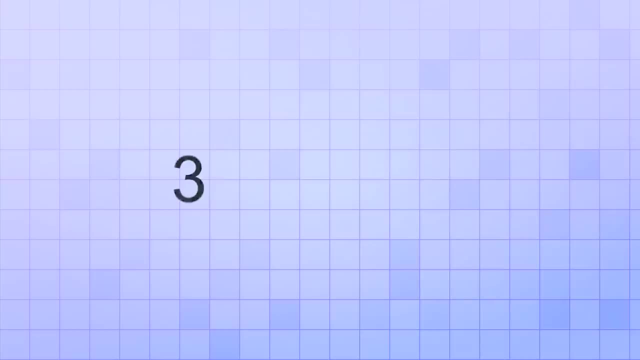 Let's look at a few examples so you see the pattern. 3% means 3 over 100.. 10% means 10 over 100.. 25% means 25 over 100.. And 75% means 75 over 100.. 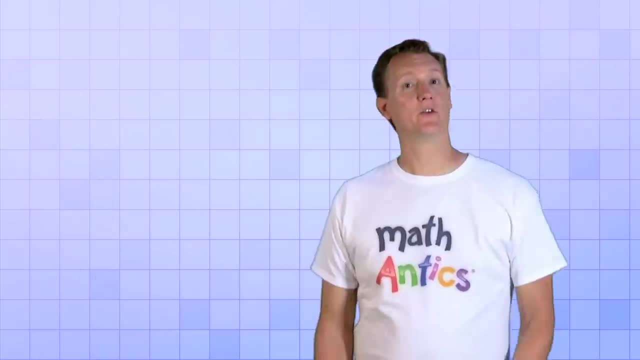 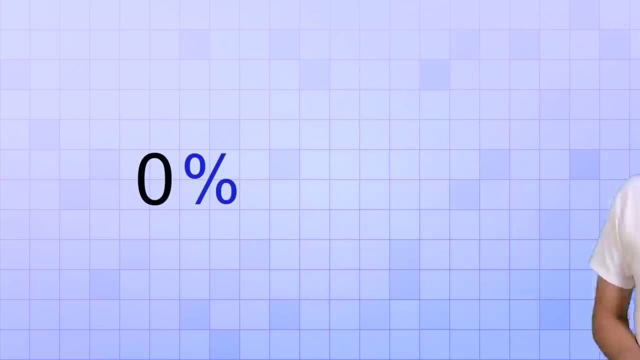 These are percents and these are the fractions that they stand for. There's a few other interesting percents that we should take a look at, Like this one: 0%. Can you have 0%? Yes, 0% would just mean 0 over 100.. 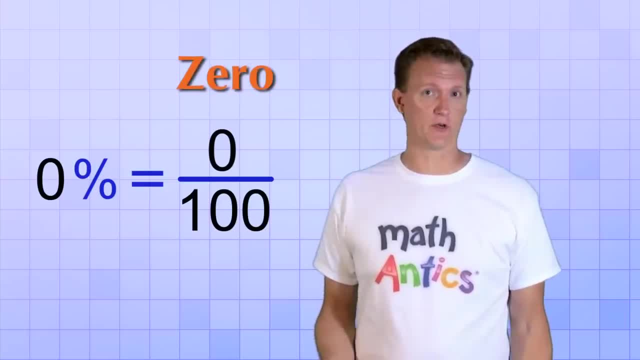 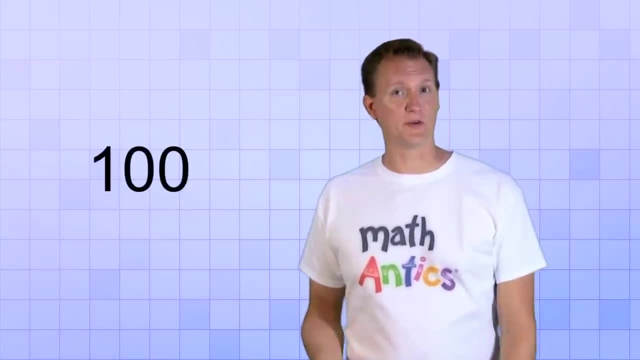 It's what we like to call a zero fraction, because its value is just zero. Remember, it's okay to have zero on the top of a fraction, but not the bottom. Alright then, What about 100%? Well, 100% just means 100 over 100.. 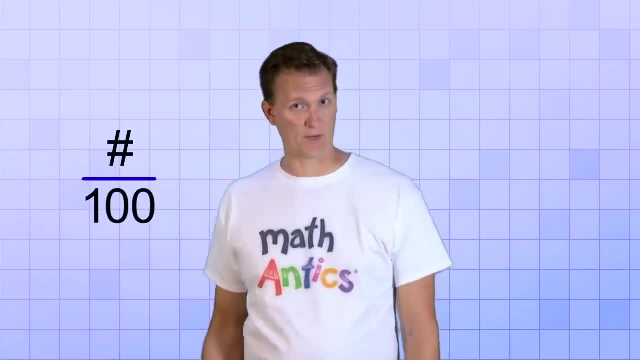 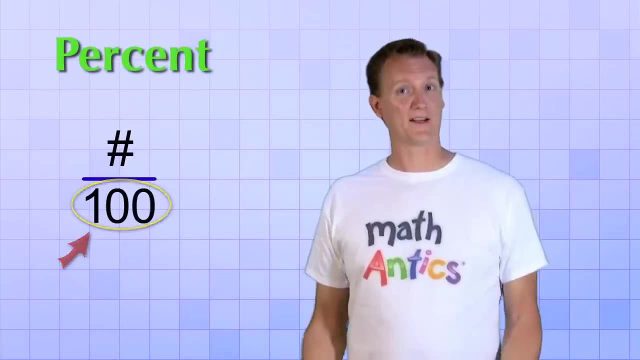 A percent is a special fraction that always has 100 as the bottom number. If it's a percent, then no matter what the top number is, the bottom number will be 100.. In fact, because the bottom number of a percent is always 100, we don't even write it. 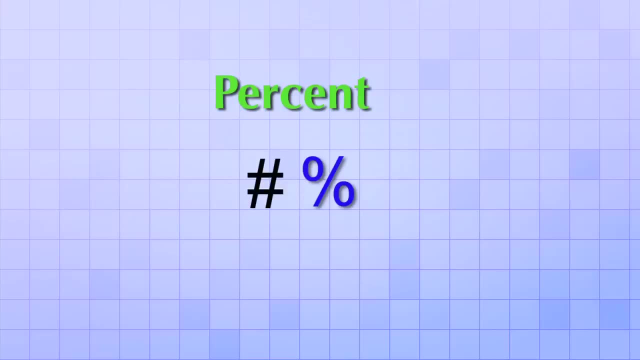 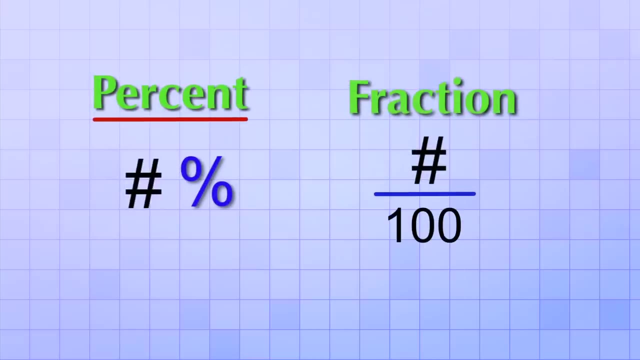 Instead, we use this handy little symbol called a percent sign. Whenever you see this symbol after a number, it means the number is a percent. It's really a fraction with 100 on the bottom, but it's just being written in this more compact form. 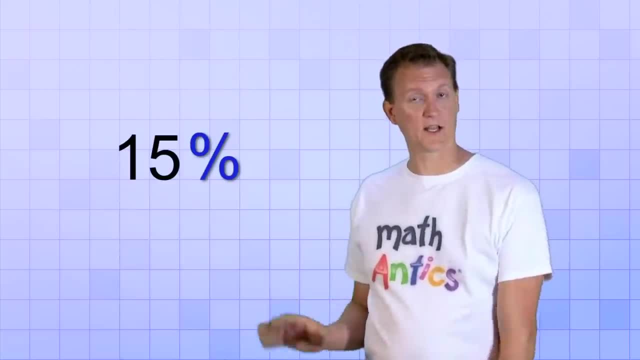 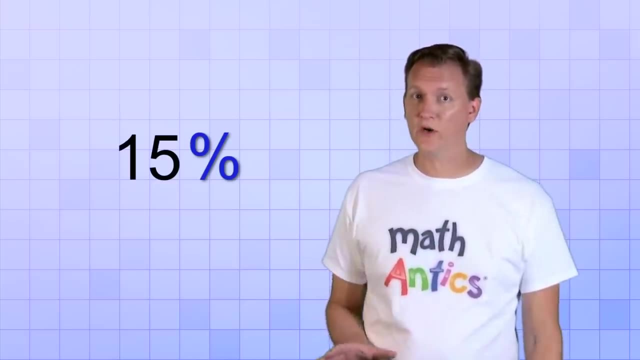 Like this number 15. here It's got the percent sign after it, so we read it as 15%, And because a percent is really a fraction that always has 100 as the bottom number, we know that it means the same thing as 15 over 100.. 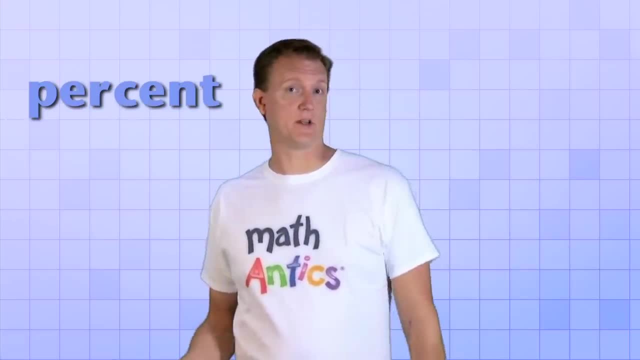 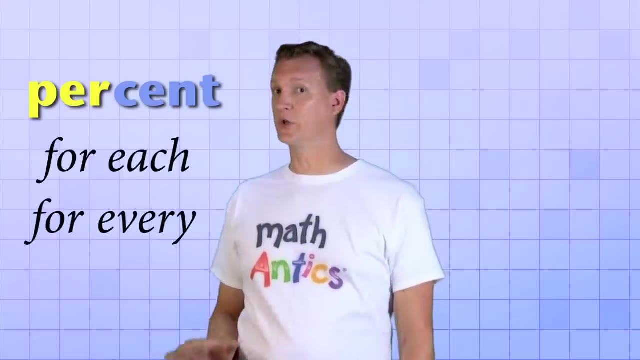 Percents make even more sense if you know what the word percent means. The prefix of the word per means for each or for every. You know like if someone said only one cookie per person And the root word cent is Latin for per. 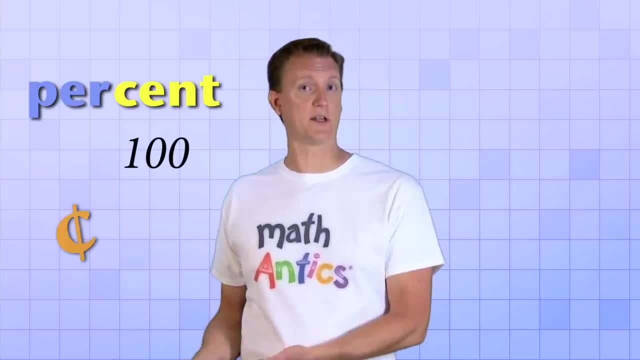 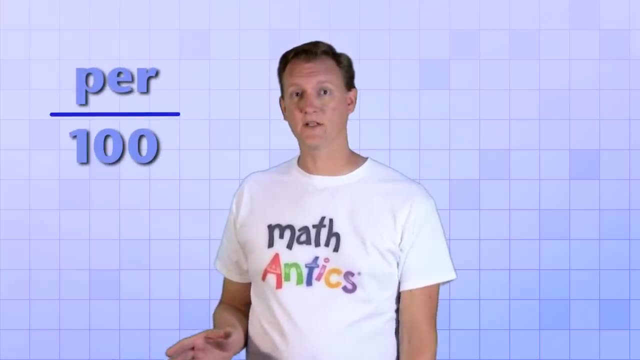 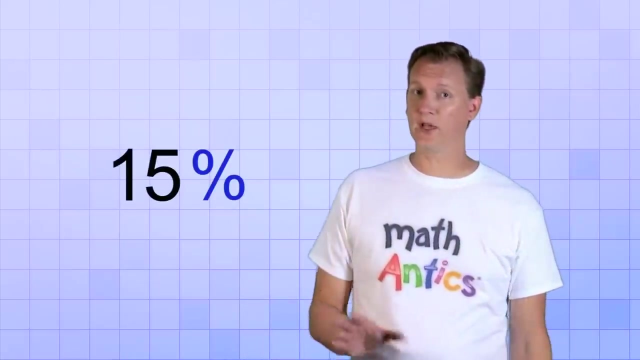 Cent is Latin for 100. That's why there's 100 cents in a dollar. So percent literally means per 100. And that's why there's shortcuts for writing fractions that have 100 as the bottom number. Alright then. So whenever you see a percent like this, you know it can be replaced with or converted to a fraction. 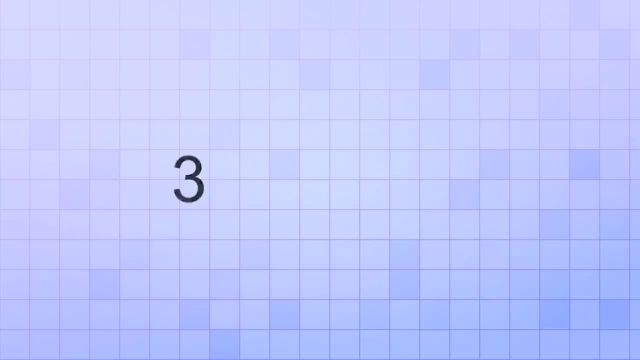 Let's look at a few examples so you see the pattern. 3% means 3 over 100.. 10% means 10 over 100.. 25% means 25 over 100.. And 75% means 75 over 100.. 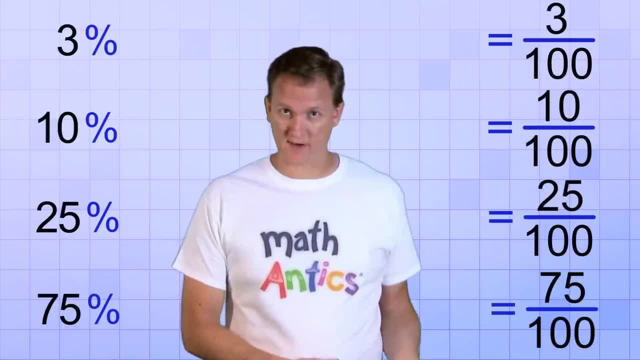 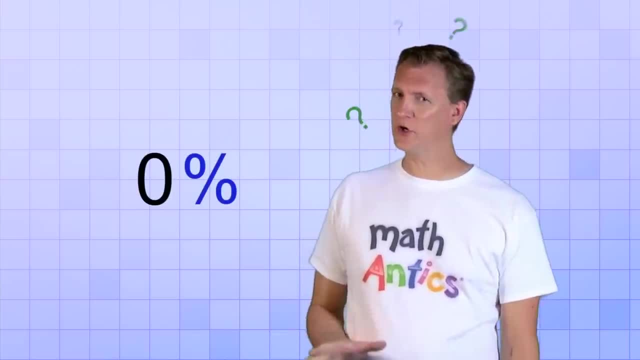 These are percents and these are the fractions that they stand for. There's a few other interesting percents that we should take a look at, Like this one: 0%. Can you have 0%? Yes, 0% would just mean 0 over 100.. 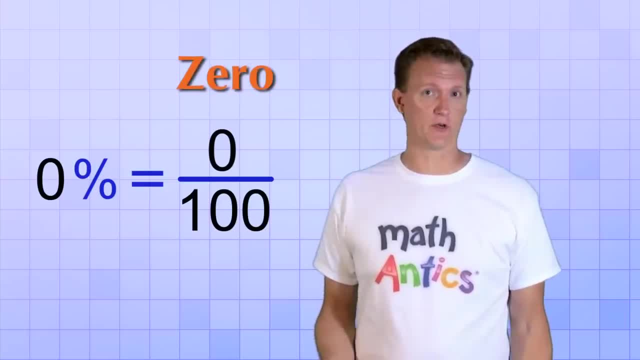 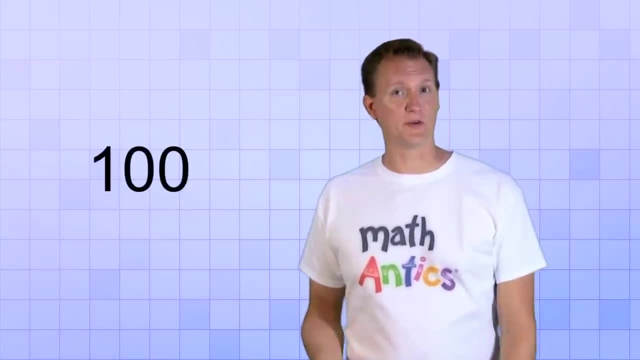 It's what we like to call a zero fraction, because its value is just zero. Remember, it's okay to have zero on the top of a fraction, but not the bottom. Alright then, What about 100%? Well, 100% just means 100 over 100.. 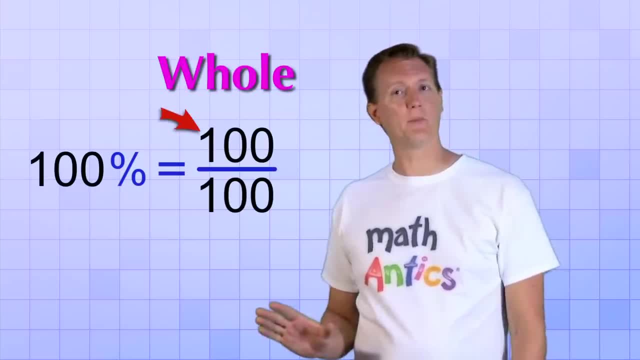 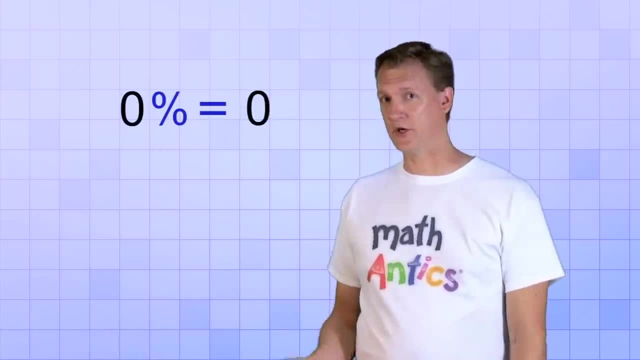 That's what we like to call a whole fraction. The top number is the same as the bottom, so its value is just one whole or one. Okay, then 0% is just zero and 100% is just one. But what about numbers bigger than 100?? 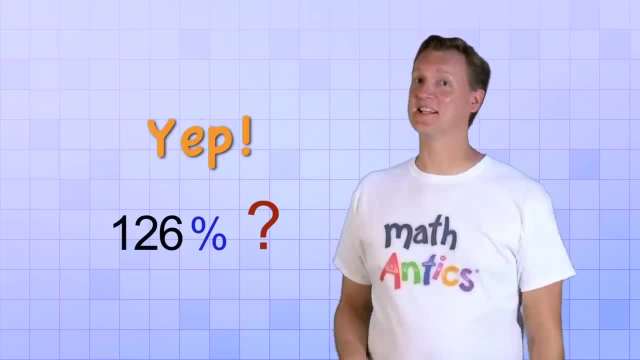 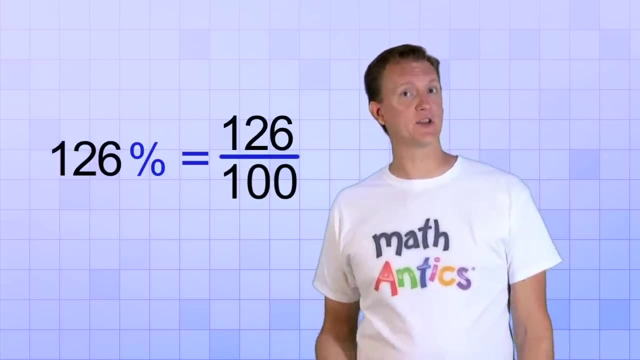 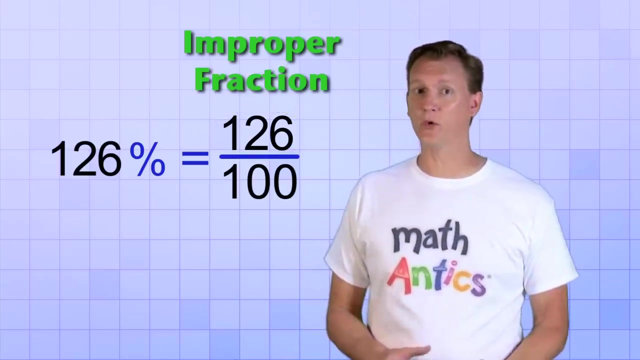 Can you have 126%? Yup, it works exactly the same way. 126% just means 126 over 100.. And you know from the fractions videos that's what we call an improper fraction. The top number is bigger than the bottom number, so the fraction's value will be greater than one. 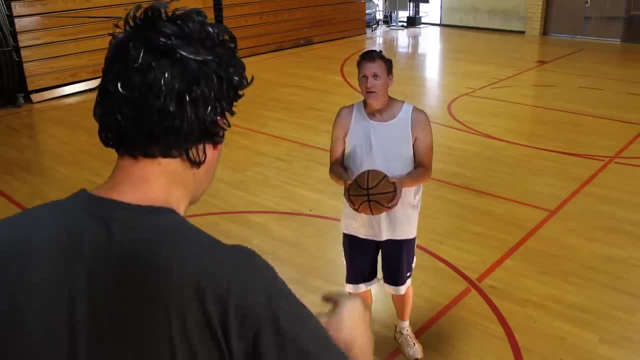 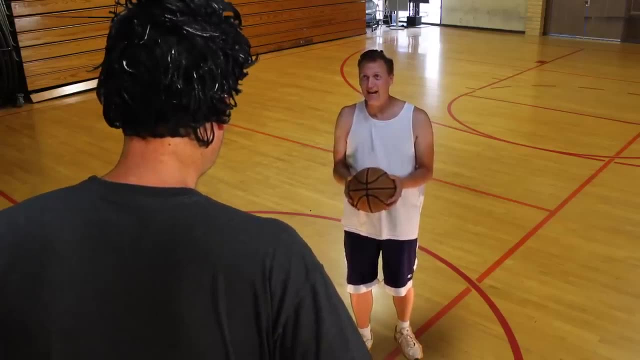 Alright team, I want you to go out there and give me 110% effort in today's game. But, coach, it would be improper for us to give 110% effort in today's game. Okay, so now you know the key to percentages. 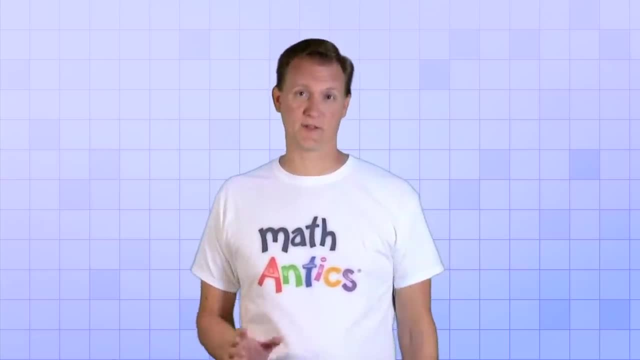 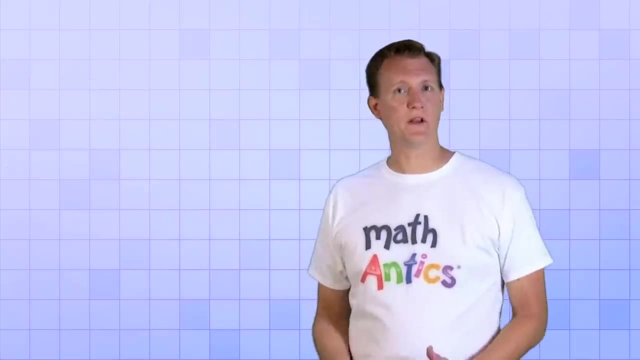 That they're just special fractions that always have 100 as the bottom number. But there's one more thing that I need to tell you about in this video, And that's decimals. Do you remember in the video about fractions and decimals that you can convert any fraction into its decimal value? 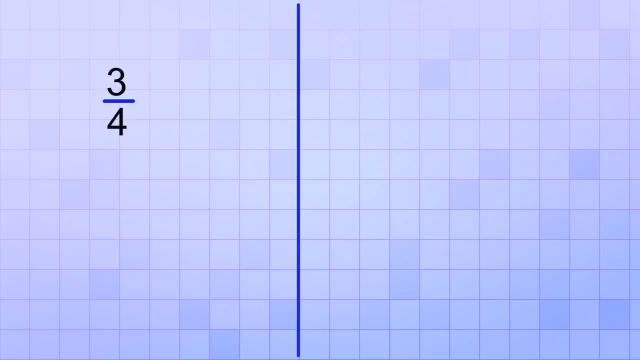 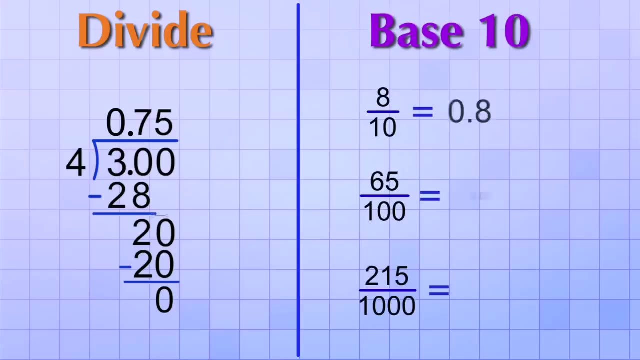 Sometimes it was kind of tricky converting to a decimal if we had to divide the top number by the bottom number. But other times, like when we had base 10 fractions, it was easy, Because decimal number places are made for counting base 10 fractions like tenths, hundredths and thousandths. 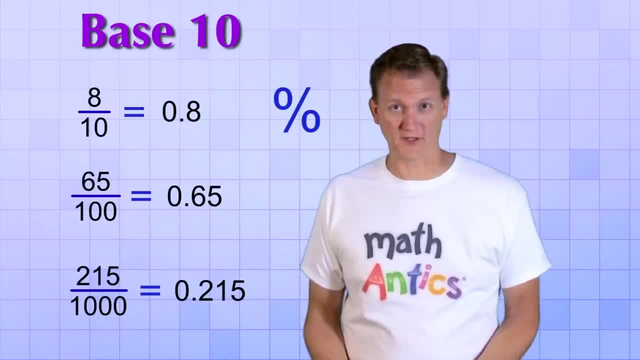 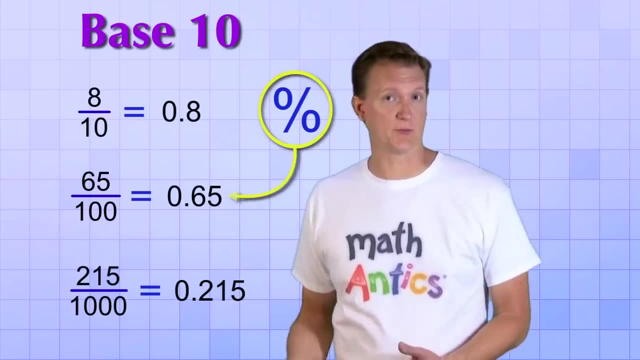 Well, guess what Percents are base 10 fractions? They're hundredths, because their bottom number is always 100. That means it's really easy to rewrite a percentage as a decimal number. You can do it the same way as we did in the base 10 fractions video. 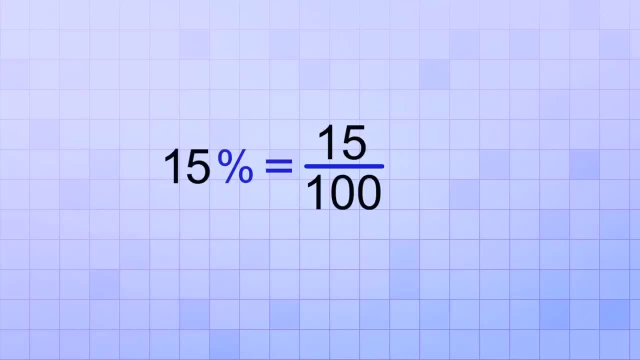 For example, we know that 15% is just 15 over 100, right, That's its fraction form, But it also has the decimal form 0.15, because this is the hundredths place and 0.15 means 15 hundredths. 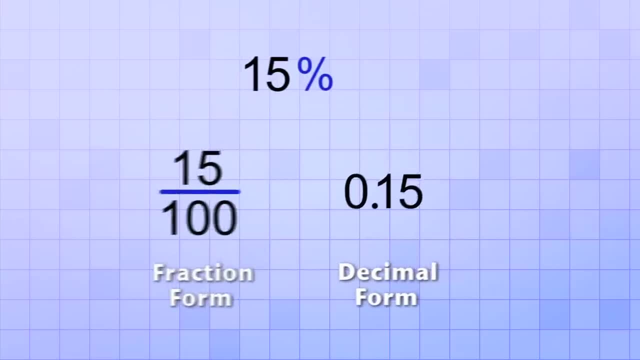 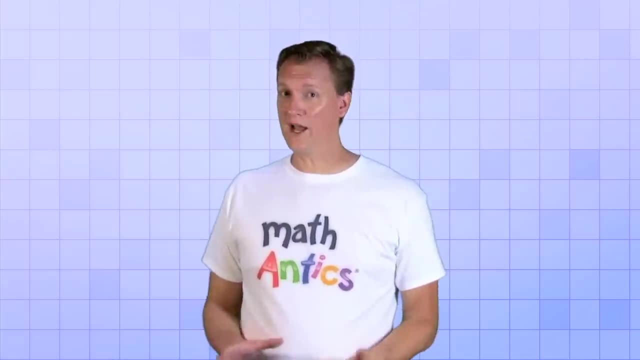 So… Now we can rewrite 15% as a fraction, 15 over 100, or as a decimal: 0.15.. And now that you know why we can easily convert a percentage to a decimal, let me show you a really simple trick for doing it. 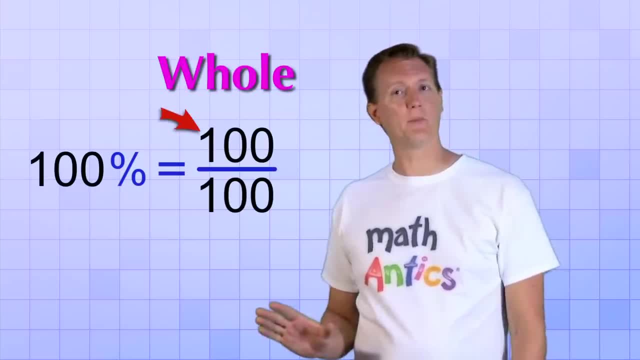 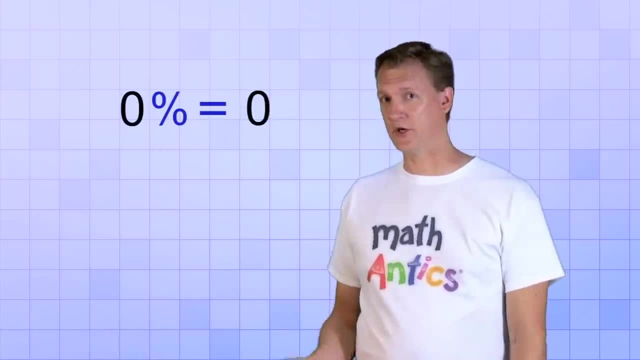 That's what we like to call a whole fraction. The top number is the same as the bottom, so its value is just one whole or one. Okay, then 0% is just zero and 100% is just one. But what about numbers bigger than 100?? 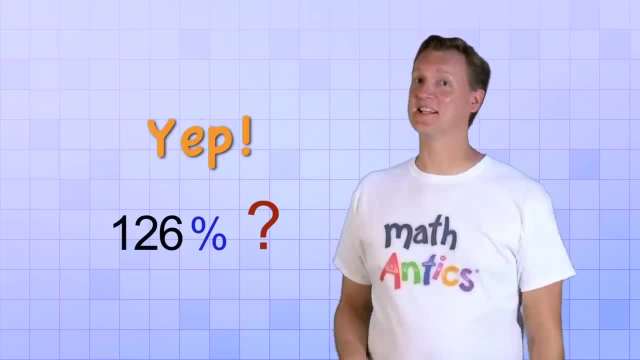 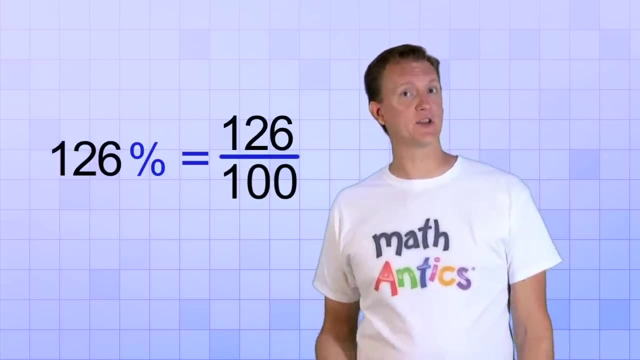 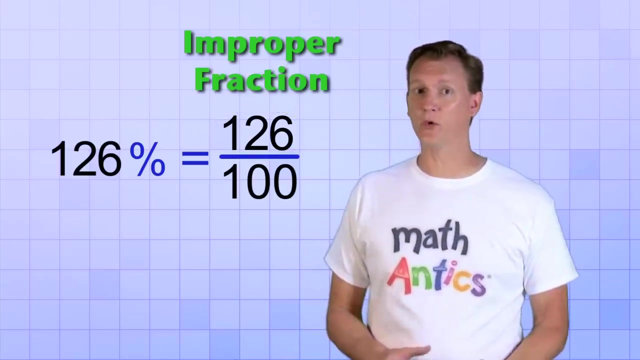 Can you have 126%? Yup, it works exactly the same way. 126% just means 126 over 100.. And you know from the fractions videos that's what we call an improper fraction. The top number is bigger than the bottom number, so the fraction's value will be greater than one. 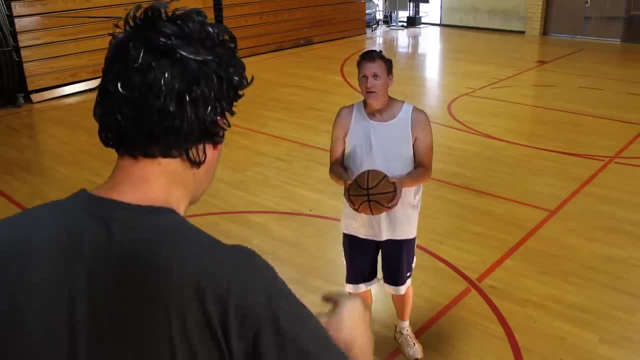 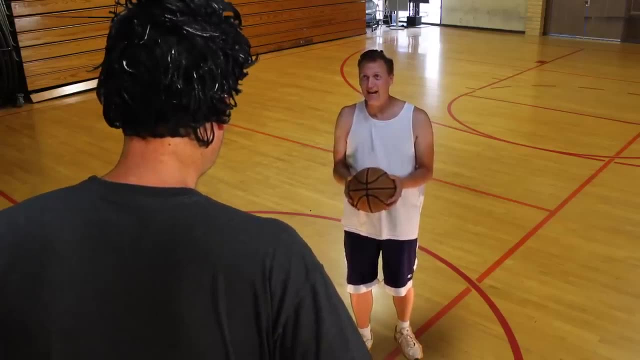 Alright team, I want you to go out there and give me 110% effort in today's game. But, coach, it would be improper for us to give 110% effort in today's game. Okay, so now you know the key to percentages. 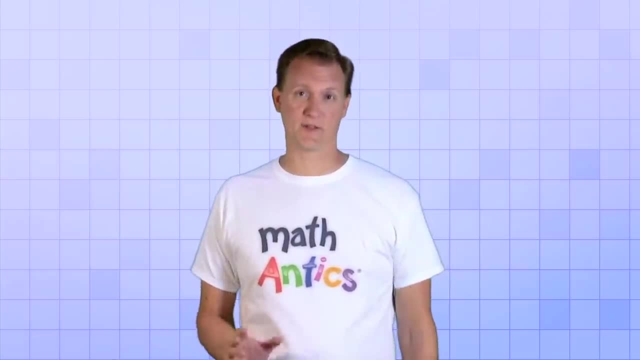 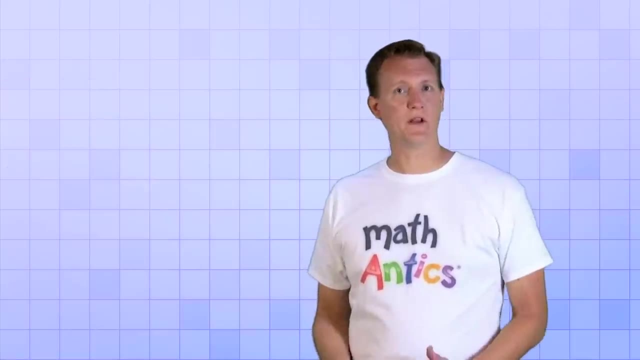 That they're just special fractions that always have 100 as the bottom number. But there's one more thing that matters That I need to tell you about in this video, And that's decimals. Do you remember in the video about fractions and decimals that you can convert any fraction into its decimal value? 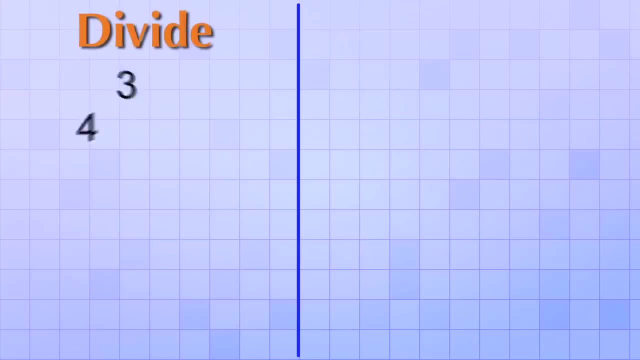 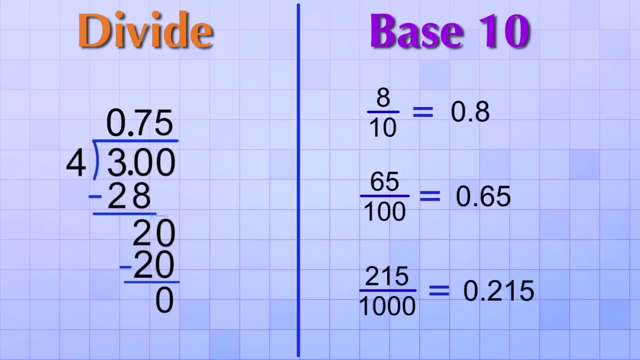 Sometimes it was kind of tricky converting to a decimal if we had to divide the top number by the bottom number, But other times, like when we had base 10 fractions, it was easy, Because decimal number places are made for counting base 10 fractions. 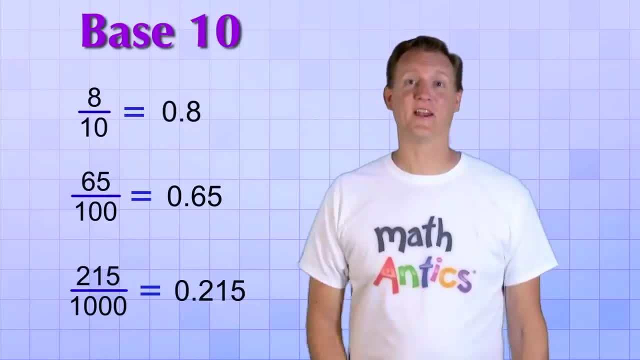 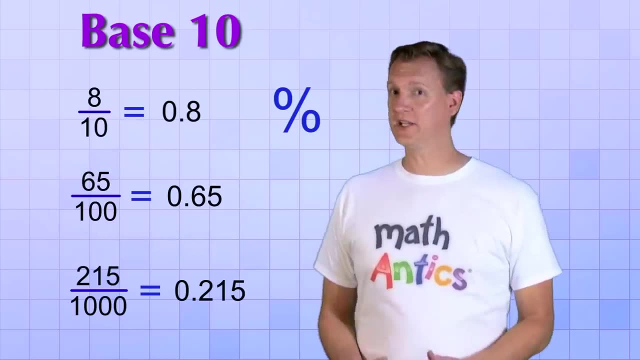 Like tenths, hundredths and thousandths. Well, guess what Percents ARE base 10 fractions? They're hundredths because their bottom number is always 100. That means it's really easy to rewrite a percentage as a decimal number. 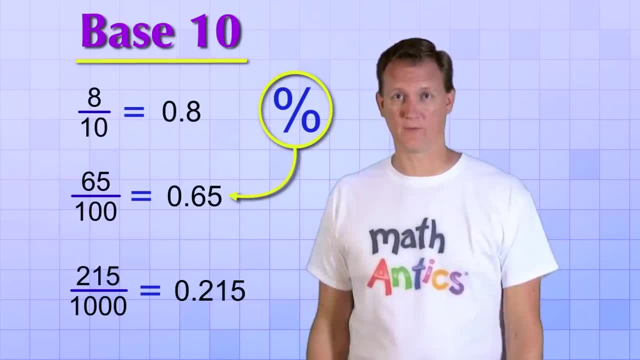 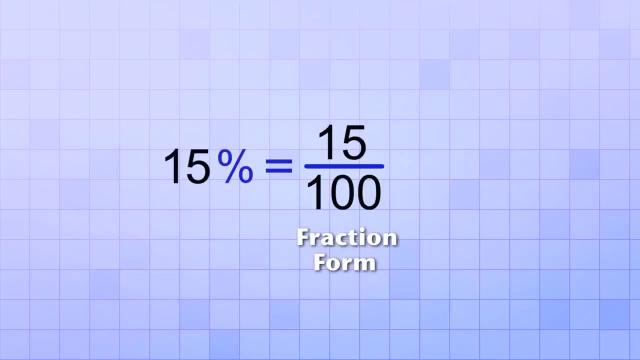 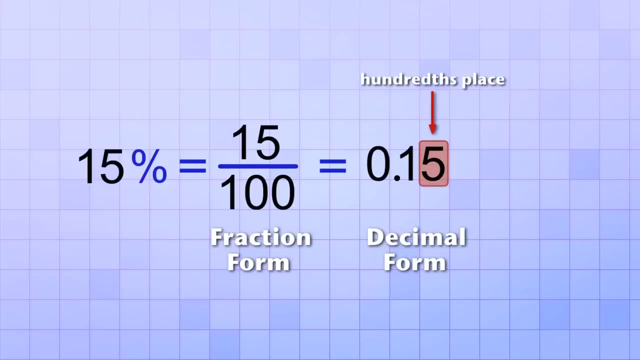 You can do it the same way as we did in the base 10 fractions video. For example, we know that 15% is just 15 over 100, right, That's its fraction form, But it also has the decimal form 0.15, because this is the hundredths place and 0.15 means 15 hundredths. 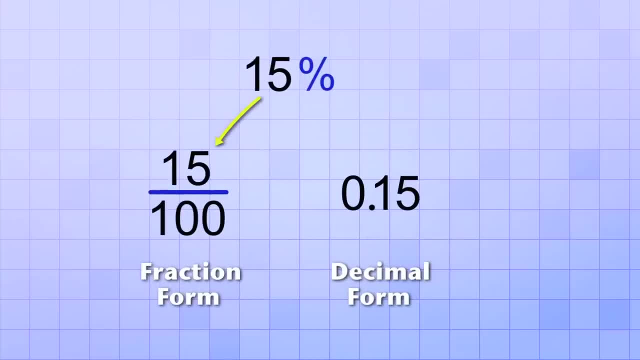 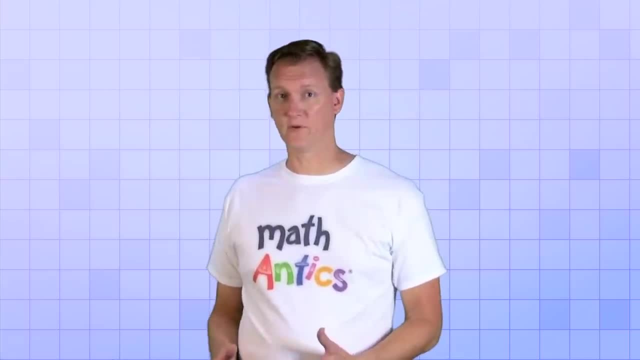 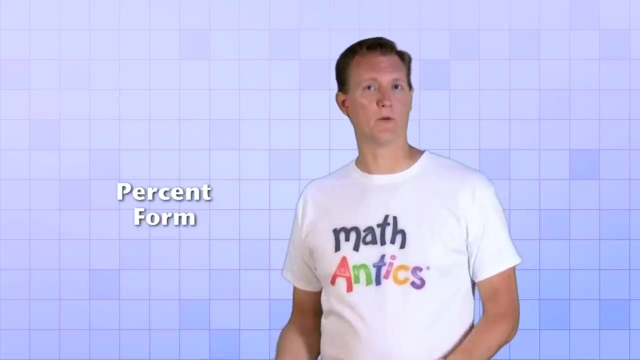 So Now we can rewrite 15% as a fraction or as a decimal. And now that you know why we can easily convert a percentage to a decimal, let me show you a really simple trick for doing it. First, you start with a number in percent form, like this: 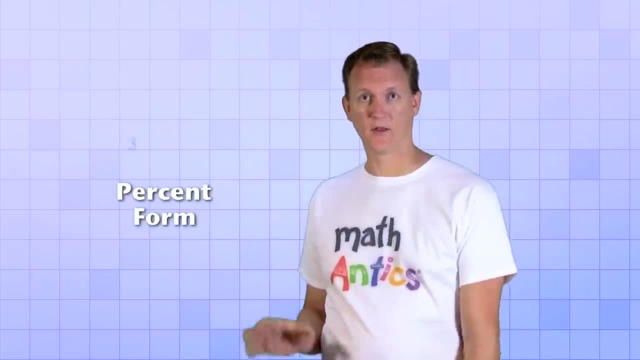 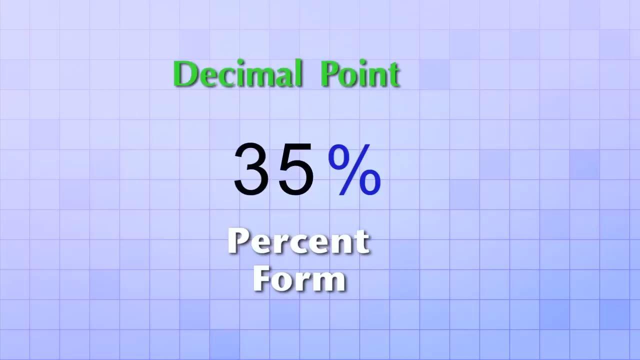 First you start with a number in percent form like this: 35%. Next you imagine where the decimal point should be in the number 35. It's not shown, but if it was it would be right here, next to the ones place. 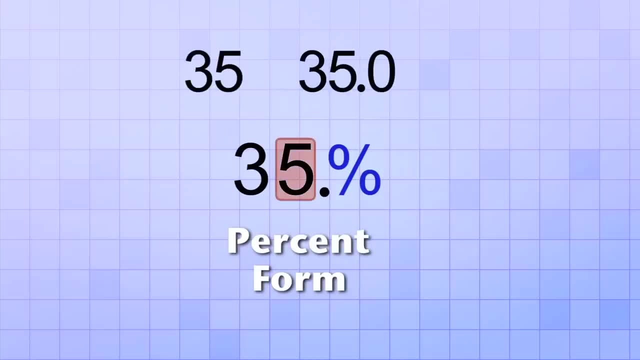 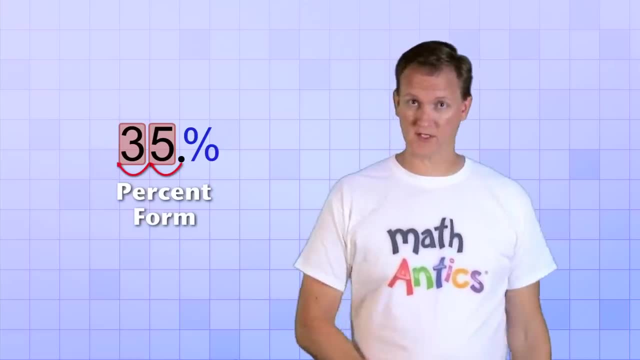 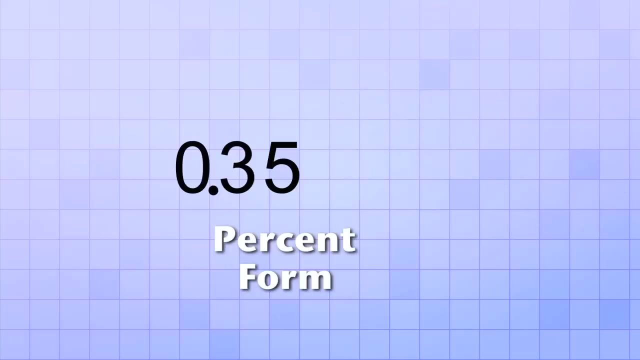 Now remember… 35 and 35.0 are the same value. Now that you know where the decimal point is, just move it two number places to the left, away from the percent symbol, and draw it in right there. Last of all, once you have moved the decimal point, you erase the percent sign because you don't have a percent anymore. 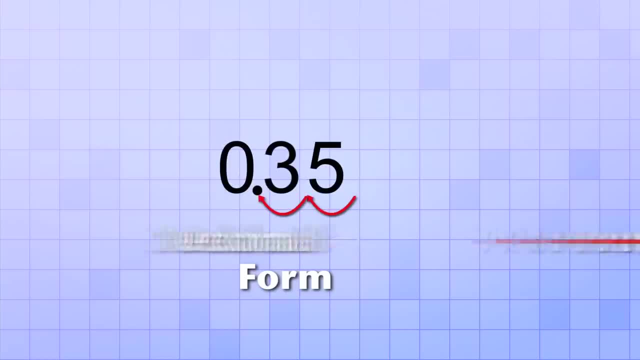 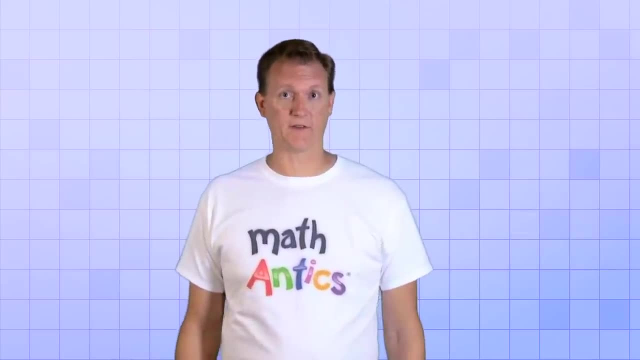 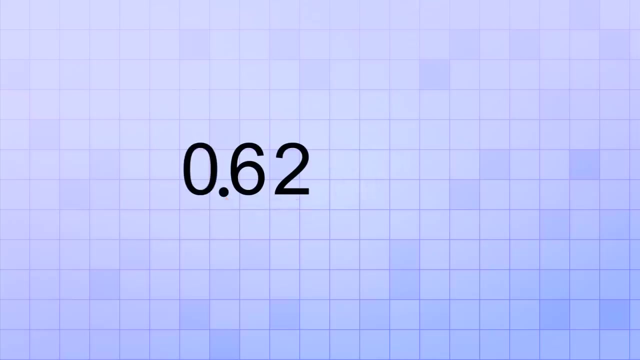 Moving the decimal point two places to the left converted it into the decimal value of that percent. Let's try converting a few more percents into their decimal values so you can get the hang of it. For 62%, we move the decimal point two places to the left and get 0.62. 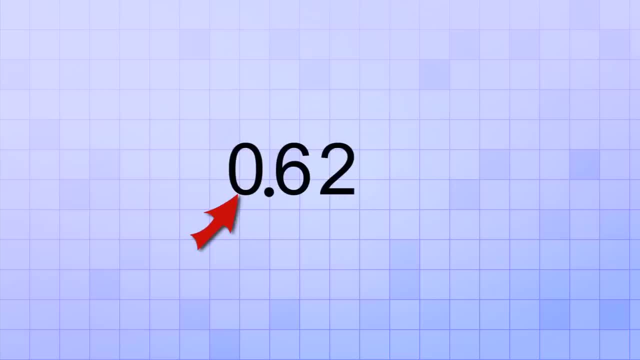 Remember, we can put an extra zero in front of the decimal point to be a placeholder and to make the decimal point easier to notice. For 75%, we move the decimal point and get 0.75.. For 99%, we move the decimal point to get 0.99. 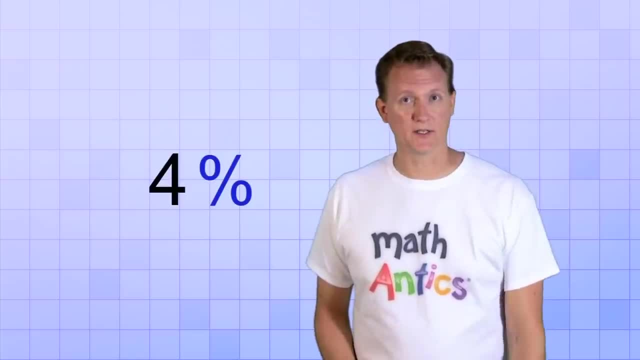 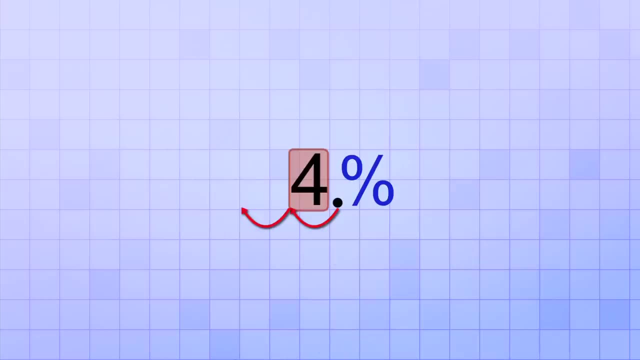 Pretty cool, huh. Okay, but what about 4%? Well, we can move the decimal point two places over when our number only has one digit, But all we need to do is use a zero as a placeholder in the number place that's missing. 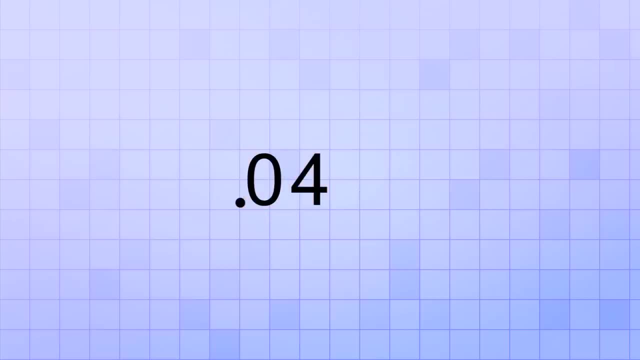 Then when we move the decimal point two places over, we end up with a decimal value of 0.04.. Now that makes sense, because 4 is in the hundredths place and 4% is 4 over 100.. 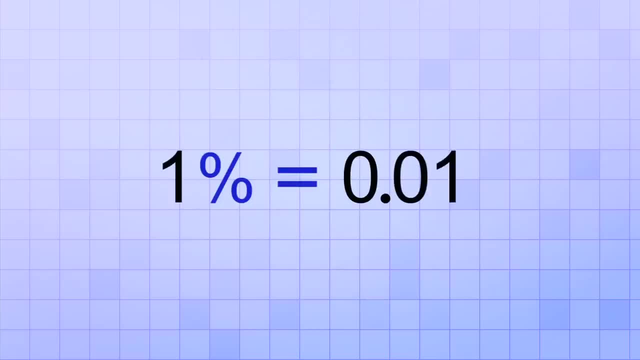 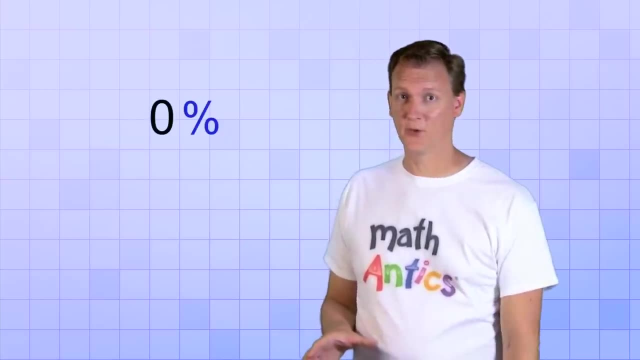 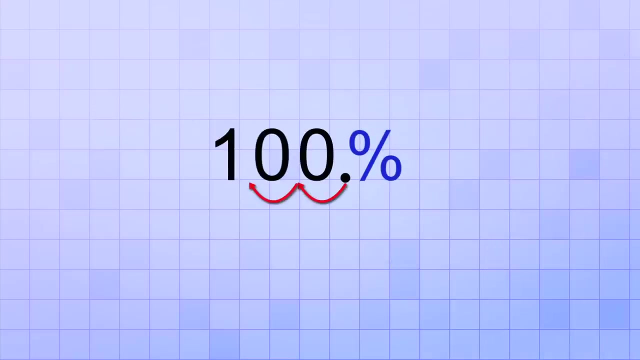 And in the same way, 1% would just be 0.01.. Again, we need that extra zero placeholder. Here's a few more interesting examples: 0% would just be 0.00.. And if we have 100% and we move the decimal point two places to the left, we end up with 1.00.. 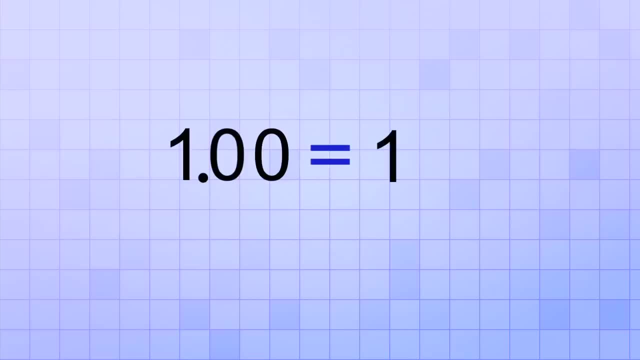 But 1.00 is the same value as 1, and that's why 100% represents one whole, And if we have 142%, we move the decimal point to get 1.42.. That's a value greater than 1,, which is what we'd expect. 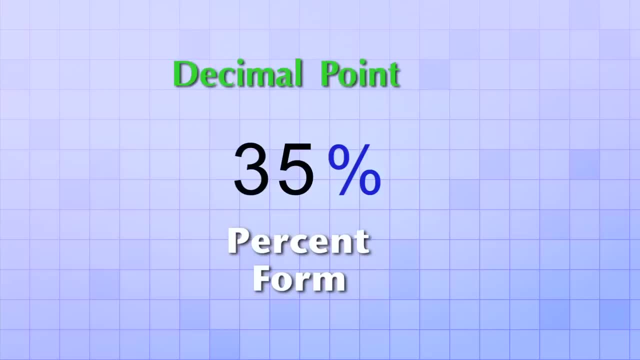 Next, you imagine where the decimal point should be in the number 35. It's not shown, but if it was it would be right here, next to the ones place. Now remember, 35 and 35.0 are the same value. 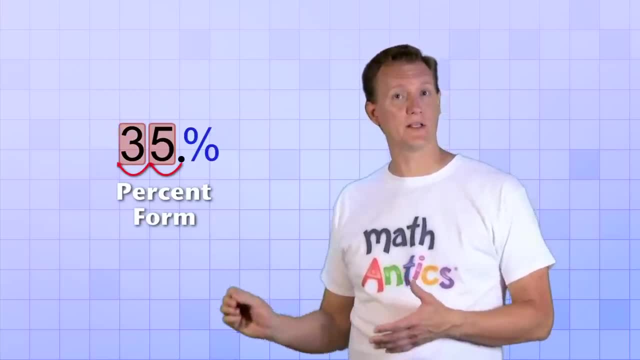 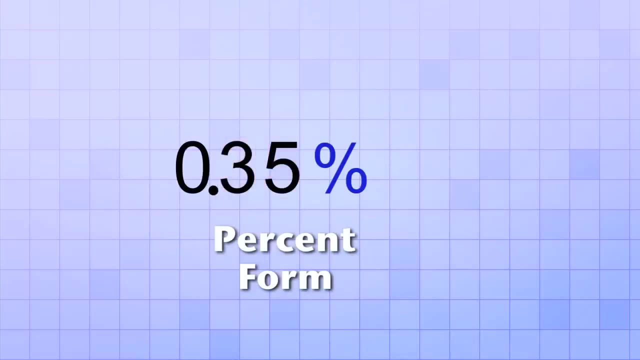 Now that you know where the decimal point is, just move it two number places to the left, away from the percent symbol, and draw it in right there. Last of all, once you've moved the decimal point, you erase the percent sign because you don't have a percent anymore. 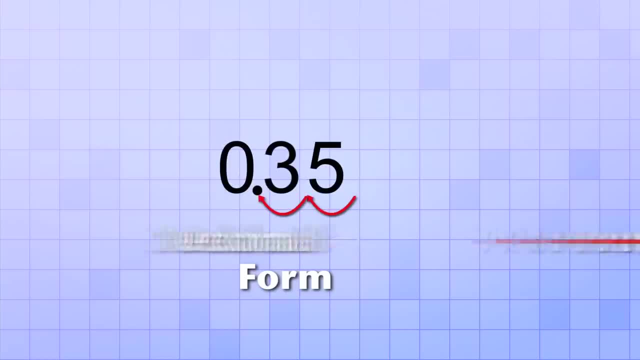 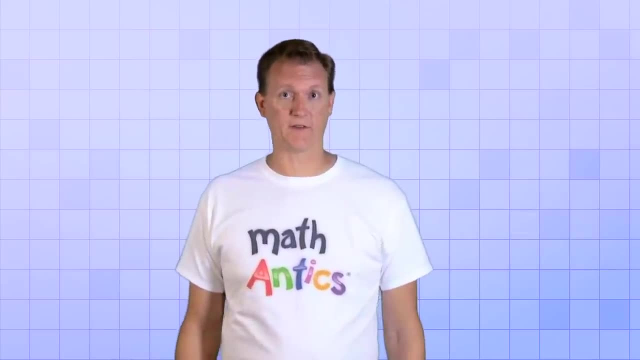 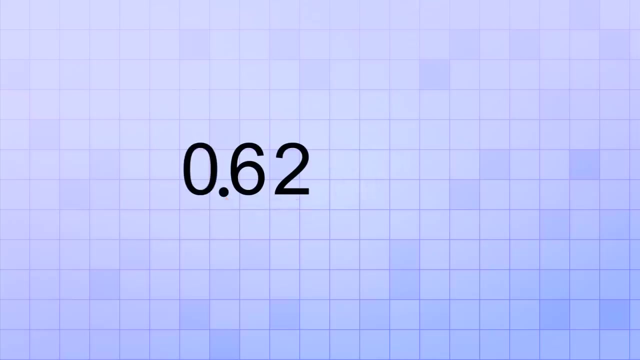 Moving the decimal point two places to the left converted it into the decimal value of that percent. Let's try converting a few more percents into their decimal values so you can get the hang of it. For 62%, we move the decimal point two places to the left and get 0.62. 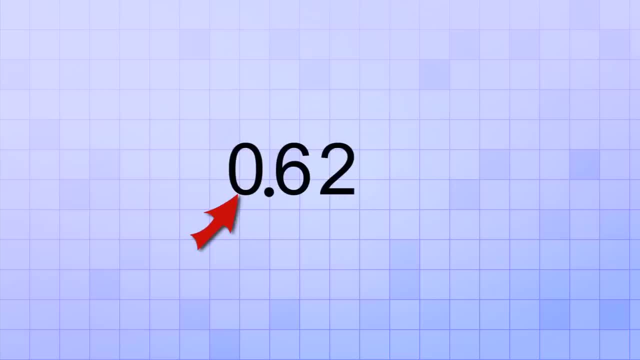 Remember, we can put an extra zero in front of the decimal point to be a placeholder and to make the decimal point easier to notice. For 75%, we move the decimal point and get 0.75.. For 99%, we move the decimal point to get 0.99. 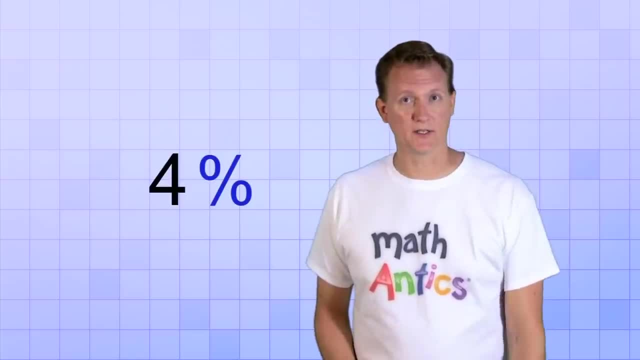 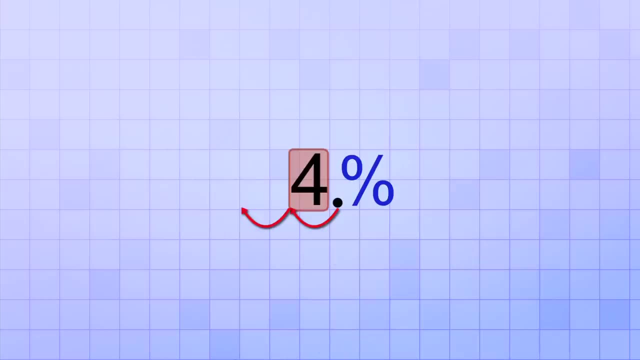 Pretty cool, huh. Okay, but what about 4%? Well, we can move the decimal point two places over when our number only has one digit, But all we need to do is use a zero as a placeholder in the number place that's missing. 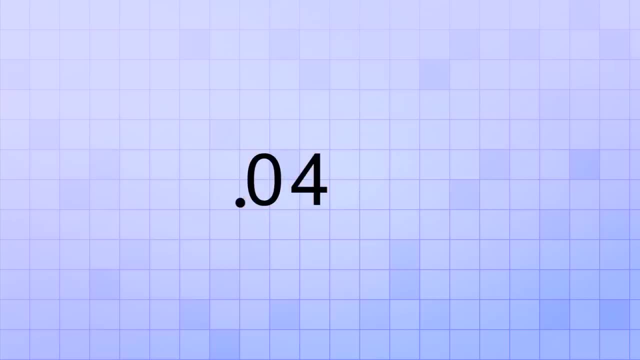 Then when we move the decimal point two places over, we end up with a decimal value of 0.04.. Now that makes sense, because 4 is in the hundredths place and 4% is 4 over 100. And in the same way, 1% would just be 0.01.. 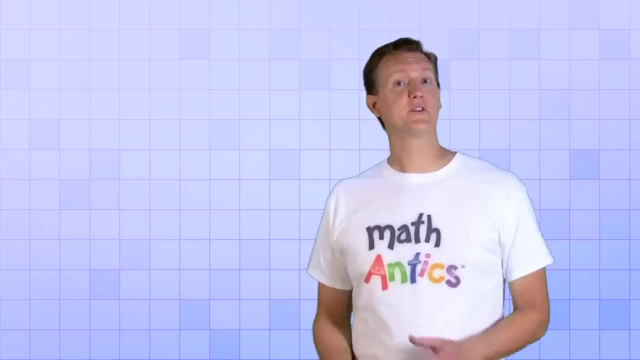 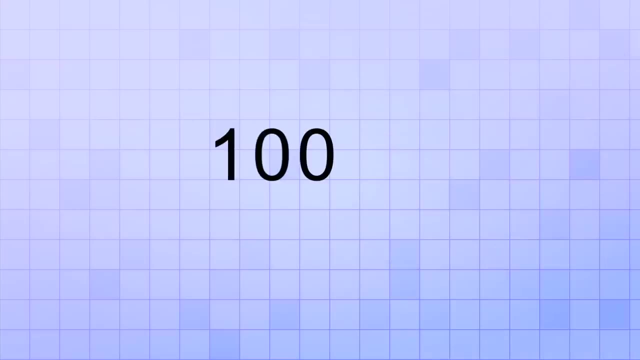 Again, we need that extra zero placeholder. Here's a few more interesting examples: 0% would just be 0.00. And if we have 100% and we move the decimal point two places to the left, we end up with 1.00.. 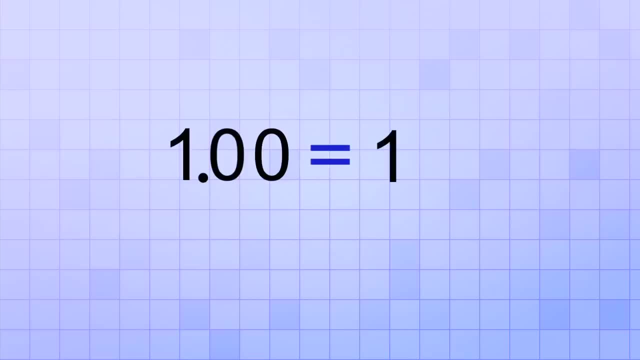 But 1.00 is the same value as 1. And that's why 100% represents one whole, And if we have 142%, we move the decimal point to get 1.42.. That's a value greater than 1,, which is what we'd expect.